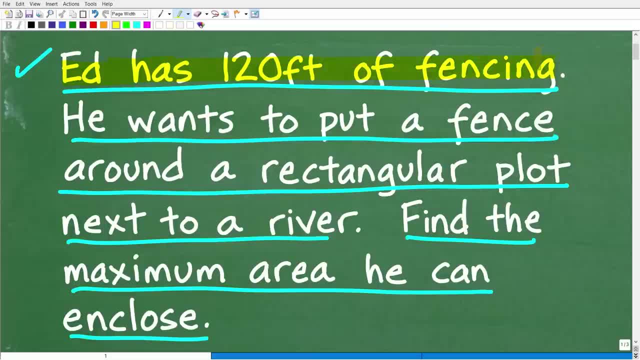 All right, now we're talking about, obviously, some sort of fence- like a chain link fence probably is the most likely scenario- And he wants to put a fence around a rectangular plot of land Next to a river. Now this part of the problem could be a little bit confusing. 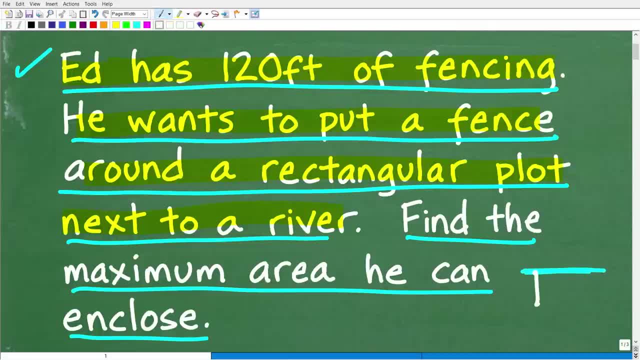 So we have a river and the fence is going to make up three sections of this rectangular plot. Okay, not all four sides, because the back of this side, right here, of what we're enclosing is the actual river right. So that's an important detail, just in case you were confused about what the problem is saying. 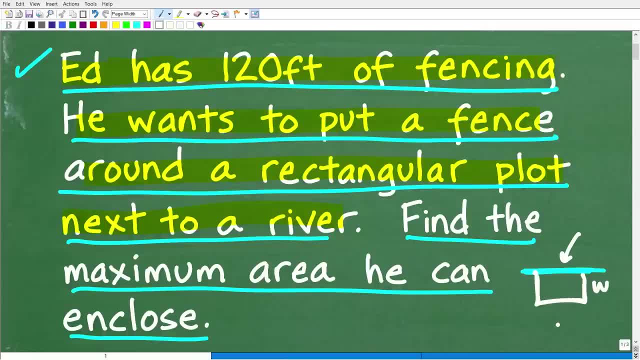 We're only talking about three sections here, but we have some sort of width and some sort of length that we need to kind of. we need to kind of make this u section of the fence with this 120 feet or ed does, but the kind of the objective here is to maximize the area that he can enclose. okay, so that obviously, 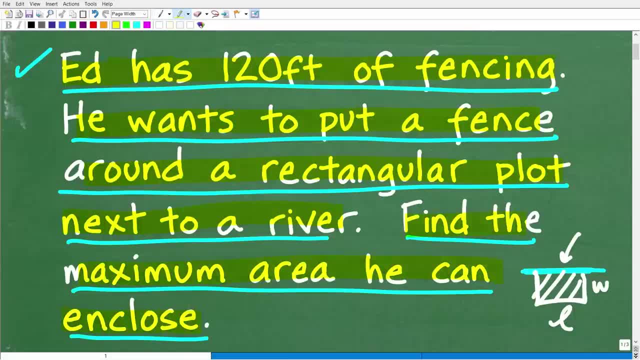 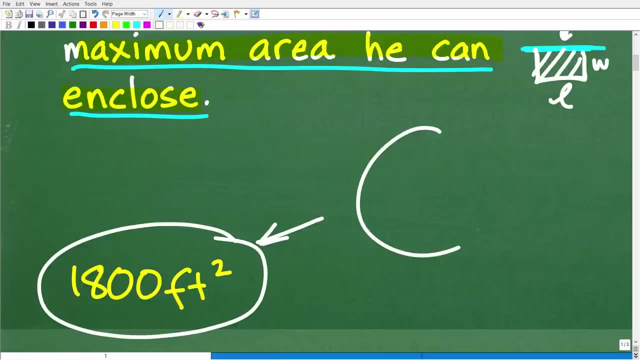 is the question: find the maximum area that he can enclose with this amount of fencing. all right, so hopefully you understand the question and hopefully you got the right answer, which is 1800 square feet. all right now. if you got this right, that is super impressive. matter of fact, i have to give you a nice. 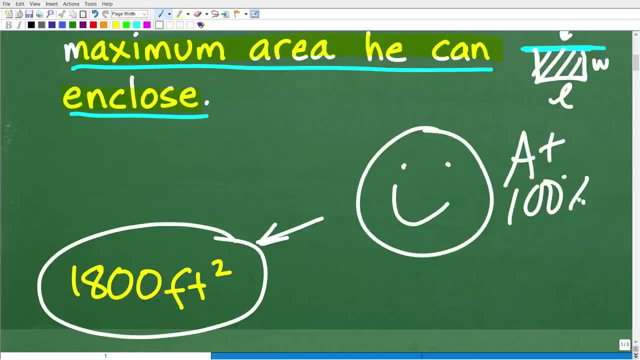 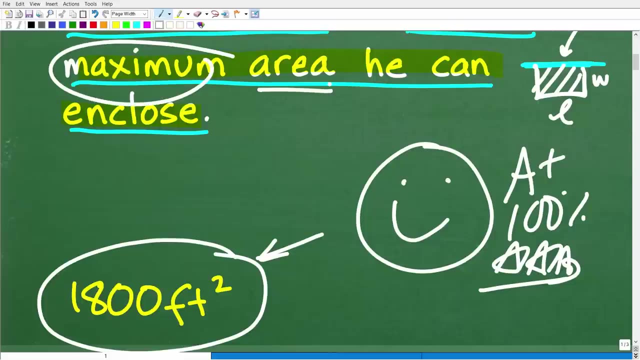 little happy face and a plus, a 100 percent and multiple stars, so you can tell your friends and family that indeed you are a certified professional expert in finding the maximum area or really kind of figuring out an optimization problem. okay, because this is what we're talking about here. 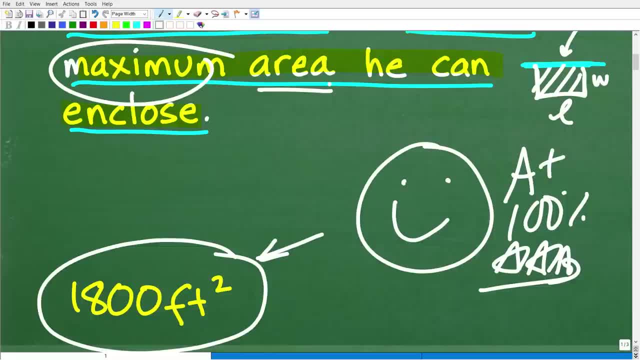 anytime you see the words maximum or minimum in a math, a problem. okay, we're talking about something called optimization, which is a big deal in calculus, but in this particular problem, you need to know a thing or two about quadratic functions, specifically parabolas. so again, if you got this right, that is super impressive, but if you didn't get this right, 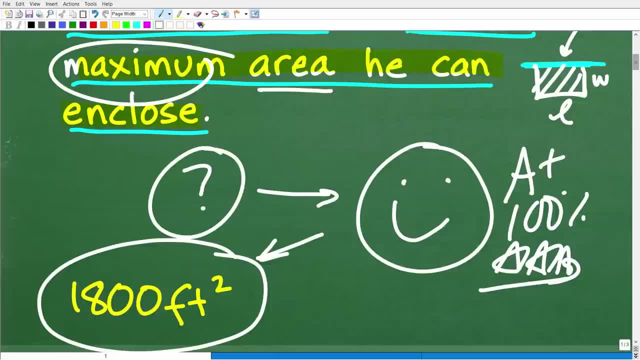 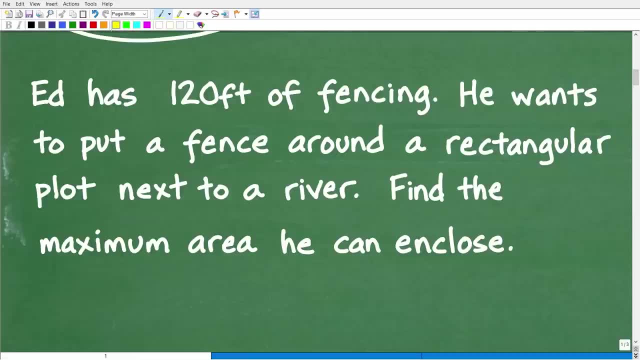 no worries, let's get into the solution right now. by the time this video finishes, you'll be a certified professional expert as well. all right, so first things first. first, we have a lovely math. one of the things that we're going to be talking about here is we're going to be talking about the 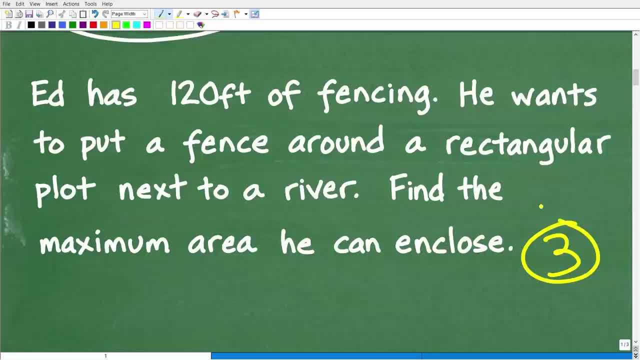 word problem: always use the rule of three. read this thing at least three times before you do anything. now i've already read it a couple times. but, um, you know, if you're confused about a problem- and let's say you are a math student, uh, taking a test or whatnot- raise your hand, say, hey, teacher, what's? 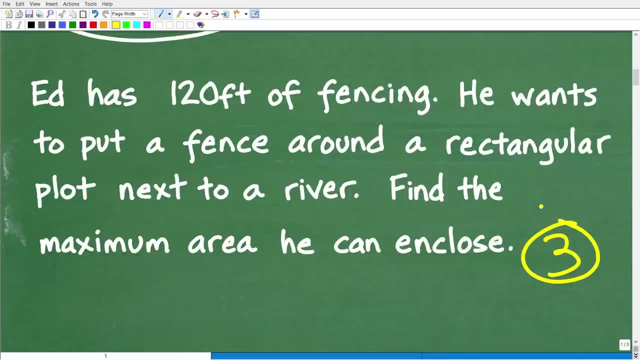 going on. i don't really kind of understand that. hopefully they'll give you some details, but if you don't understand a problem, you're not going to be able to solve it right. so this particular part about this fence- a rectangular fence next to a river- could be kind of a problem. but if you're 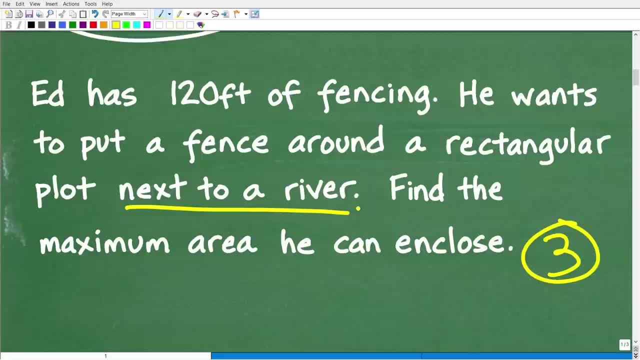 confusing, but the best way to kind of really make sure you're clear on the information in the problem is to try to model it okay, and in this case we can certainly come up with a nice, lovely sketch that represents what's going on. all right, so let's go ahead and take a look at my little. 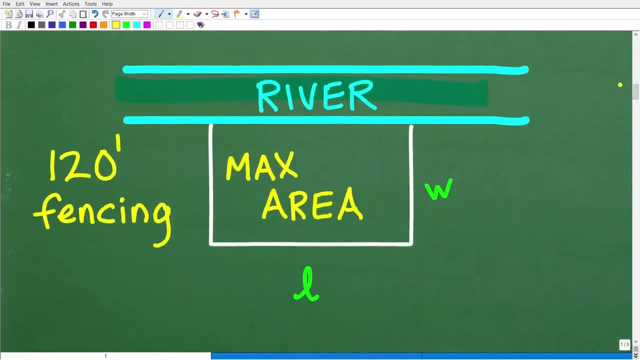 picture and here we have this river. okay, now we have 120 feet of fencing and, of course, we have this rectangular plot that we want to enclose. now, again, the river is going to be a rectangular plot. the river is going to be the back of this uh enclosure. right, so you know, we don't need uh you. 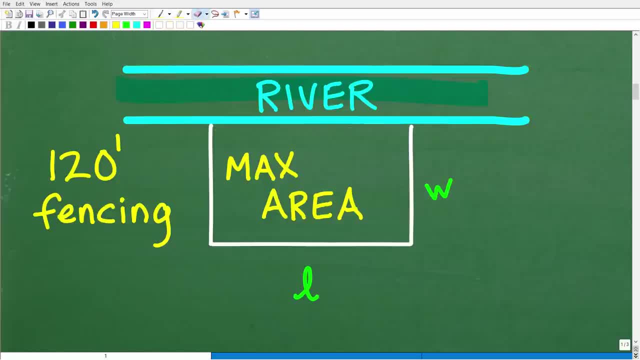 know this kind of other fence part right there. so we have three sections to make up from this, 120 feet of fencing. now the maximum area is going to be the width uh times the length, right, because the area of a rectangle is length times width. so we need to figure out the maximum area now. you might. 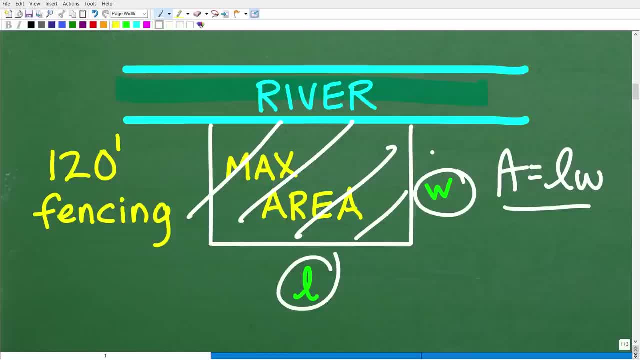 be saying to yourself: well, 120, uh feet, you know, maybe you could just put two equal parts of the equal sides here a little bit here. maybe it's not going to make a difference. well, it actually makes a big difference in terms of what width and length you use here. okay, matter of fact, let's go ahead. 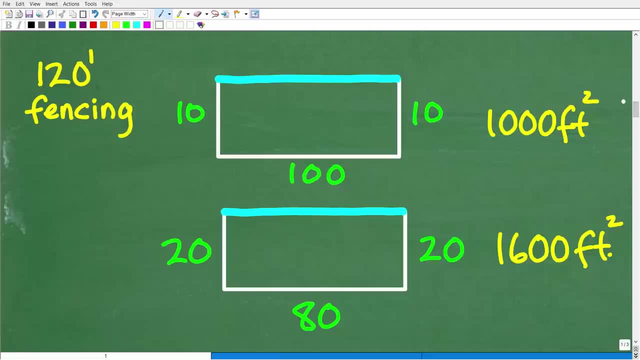 and take a look at some examples. all right, so if i have an, if i have 120 feet of fencing and let's suppose we want to kind of uh, configure our fence in this manner, okay, again, this back part of this rectangular plot is the river, so we're only talking about three sections, but we could split up this. 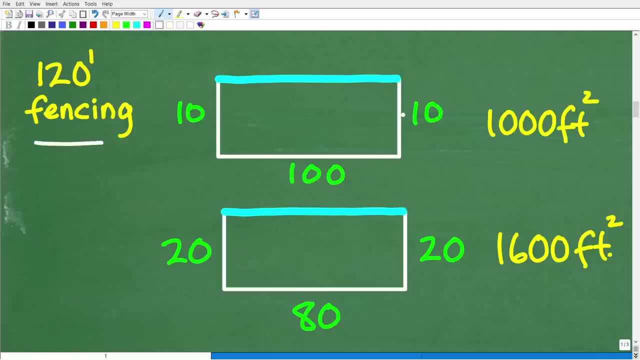 120 feet. this way, we could have 10 feet of fencing and we could have 120 feet of fencing and we could have 10 and 10 feet. remember, we are dealing with that rectangle, so these sides the widths are the same, so we're going to have 10 and 10, and so that's, of course, 20. that leaves us with 100, right. 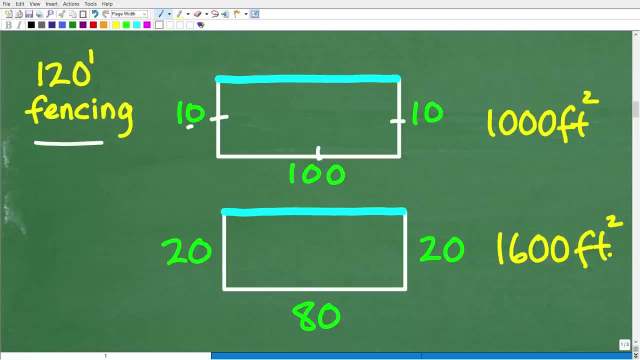 here for a grand total of 120, uh, in terms of our how much fence we have. so the area is 100 times 10, okay, which is a thousand square feet. that seems pretty good, but can we do better? well, maybe let's increase the width and then maybe we'll kind of decrease the length. so 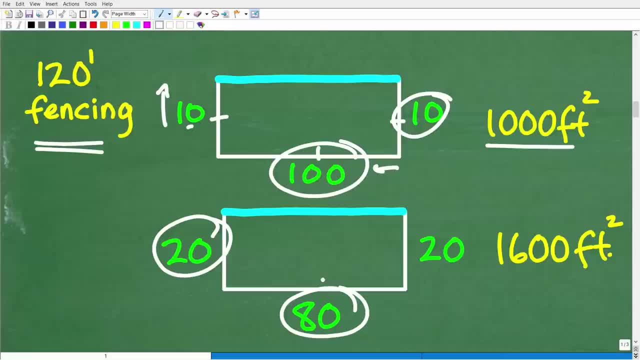 let's say we have 20 by 80. well, 20 by 80, if we get the area there, we're going to have 1600 square feet, so definitely better. so again, there is a specific- okay, uh- configuration where we have the maximum amount of area. so what are these numbers? what is the best width and length to max out the? 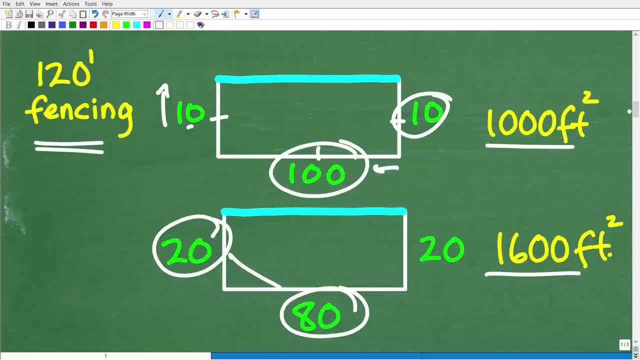 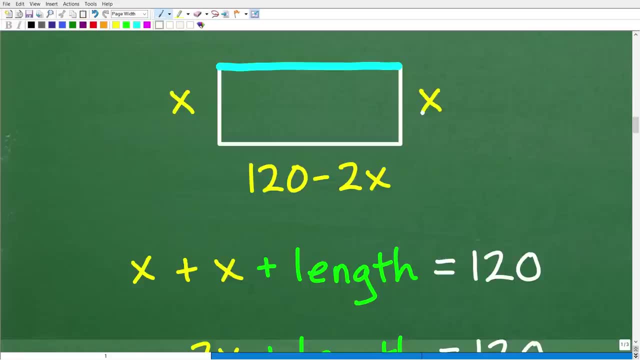 area here. well, this type of problem again is called an optimization problem. all right, but we're going to be using an optimization problem and we're going to be using an optimization problem- algebra- and what we're going to do is we're going to let this variable x represent the width of our 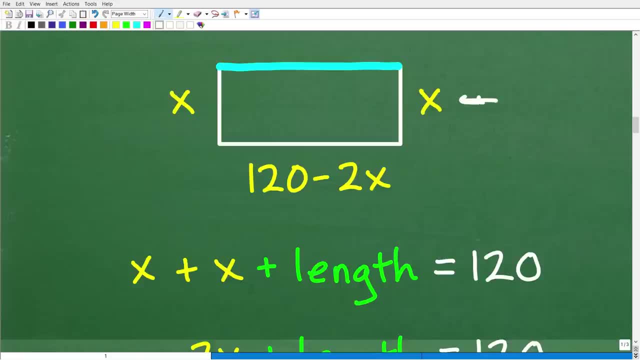 rectangular plot. okay, so if we have x over here, because this is a rectangle, we have x right here and the length is this expression right here: 120 minus 2x. now, why is that? okay, a lot of you might be saying. come on, mr youtube, math man, uh, you know, i'm a little lost. what is where is that 120? 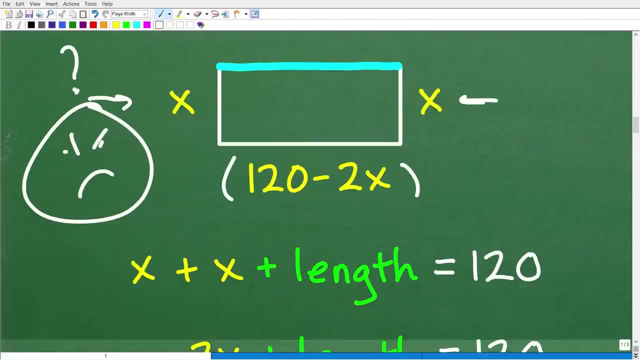 minus 2x coming from. well, let's go ahead and figure that out right now, because this is important. okay, so let's suppose- uh, we don't know how to express this length right where this is the width, this is the length of this rectangle, but we do know that this x the width and this x plus the 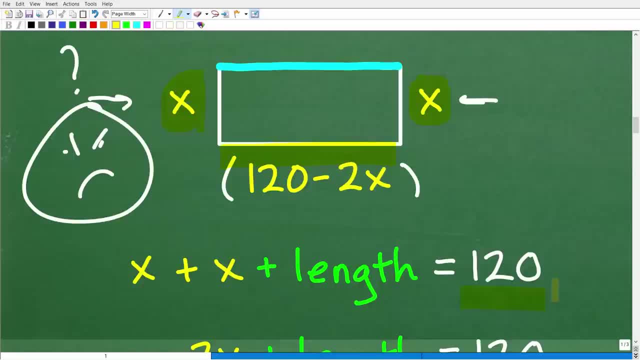 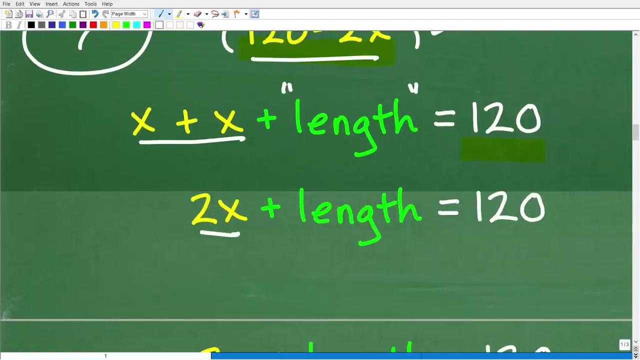 length, right, the width, and this width and this length has to add up to 120, so we have x plus x plus the length. okay, which is this right here is equal to 120, so we could kind of just solve for it, okay. so we're going to take this that equal 20 minus x plus x plus, next, y raised plus plus and. 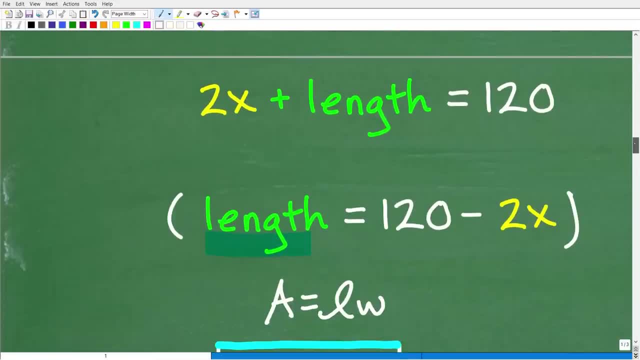 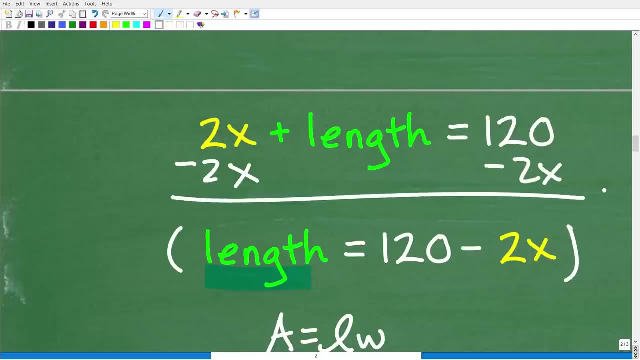 then the권 second term we're going to remember is квw is talking about right now. so we come over to the left and then we're going to try to get into the host a plus the length, which is 120 minus 2x, and the length, since we're going to get there with these rectangles, start elongating. 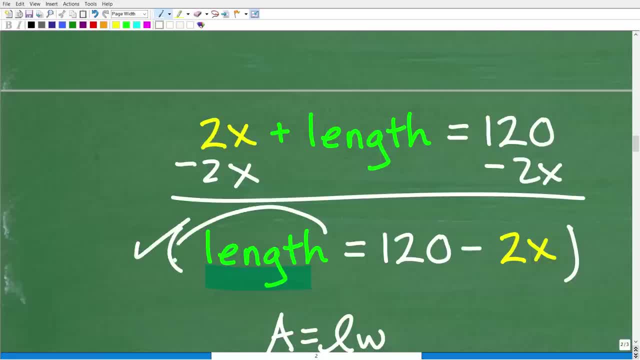 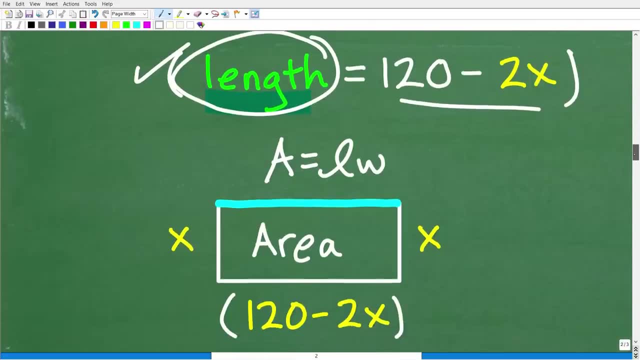 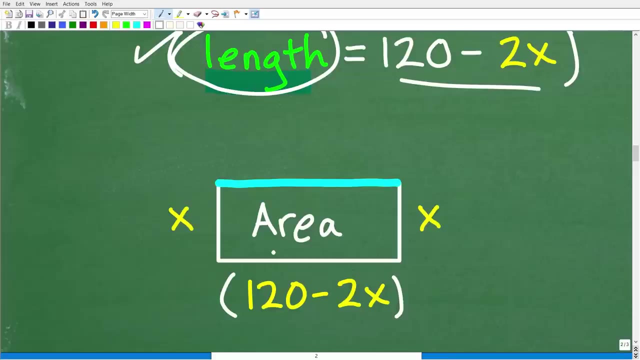 well, this a is equal to 220 minus 2x. rectangle. is this expression right here? 120 minus 2x. so that's how we come up with our 120 minus 2x. all right. so again, what we want to do here is find the area now of this enclosure and the area 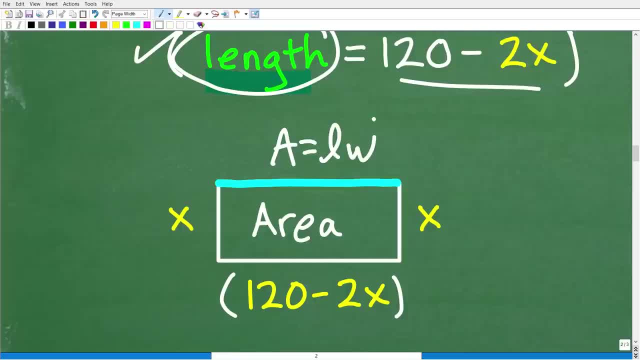 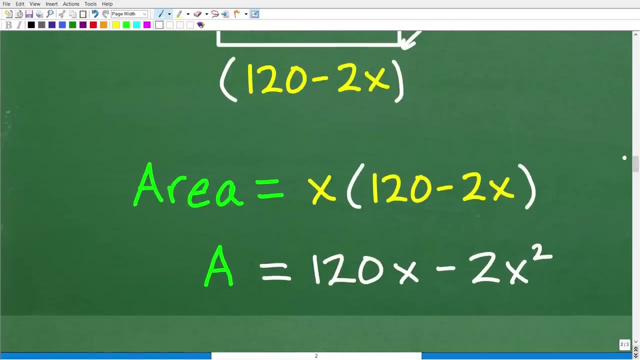 is equal to the length times the width. so in this case it'll be x times 120 minus 2x, all right, so we need to kind of maximize this. so let's go ahead and take a look at what we have here. so the area of this enclosure and we can have this algebraic variable model, x times 120 minus 2x represent the. 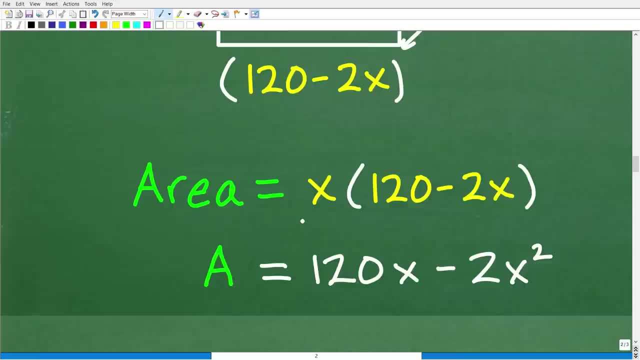 area, okay, of this particular enclosure. what we want to do here is find the. we want to maximize this. okay again, max maximization or minimization, is a part of a broader topic called optimization, which is all over the place in math, and this is where this problem is going to start getting very 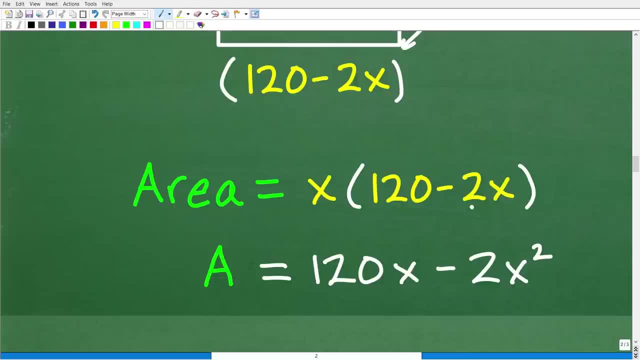 interesting, all right. so area is equal to x times 120 minus x. let's go ahead and distribute this x in, so we have x times 120, that's 120 x, x times minus 2x. so that's minus 2x squared. all right, so let's go. 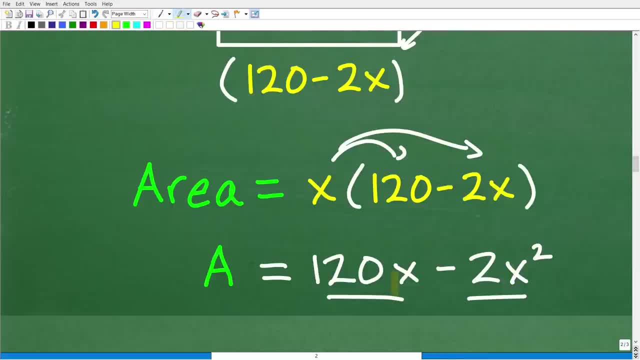 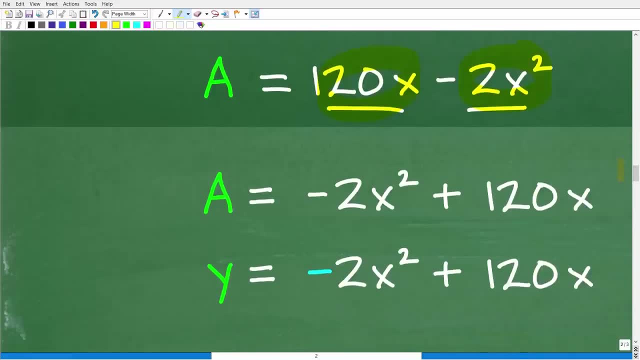 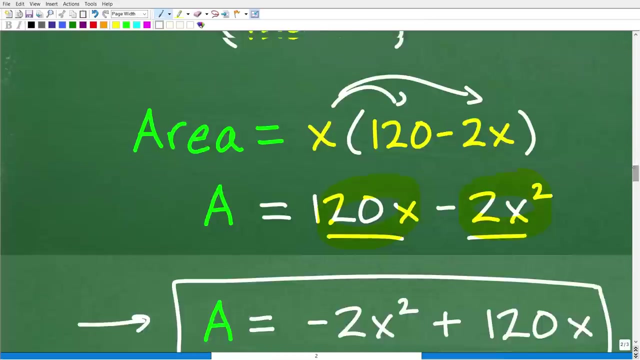 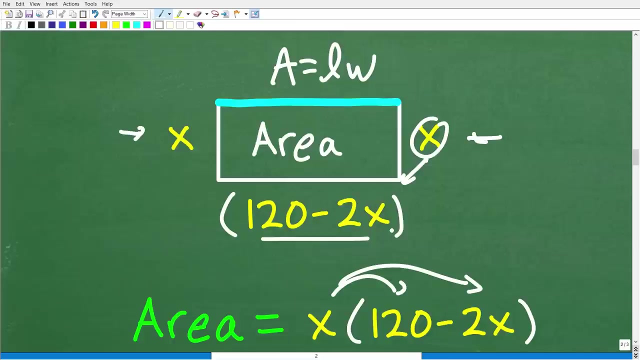 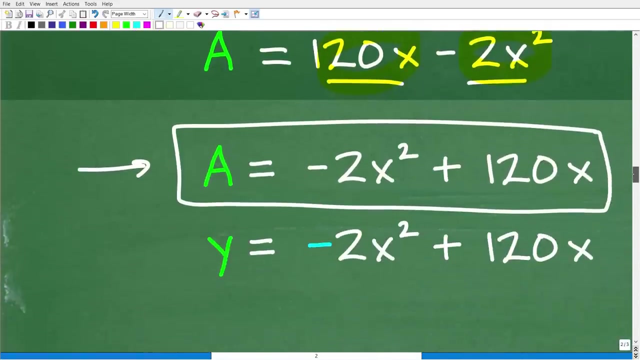 ahead and clean this up. anytime you have an x squared or x or any kind of polynomial, always write it in standard form, highest to lowest power. so that's going to give us area is equal to minus 7 or 8, and leave the negative sum on theningseka itself. we'll show you some of the profit, Ki. 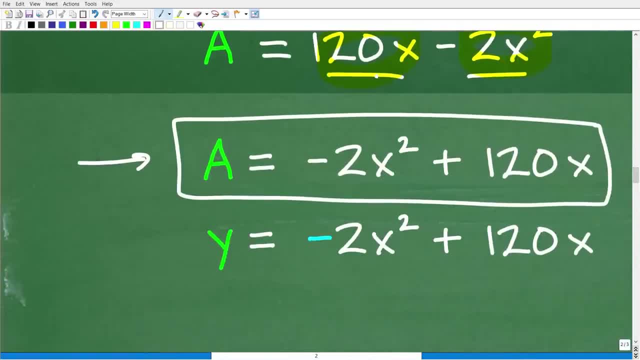 is exactly cebcaric. a is the area right. we just multiplied the length times the width. but what I'm going to do is I'm going to use a different variable for a. I'm going to use y. okay, so we have: y is equal. 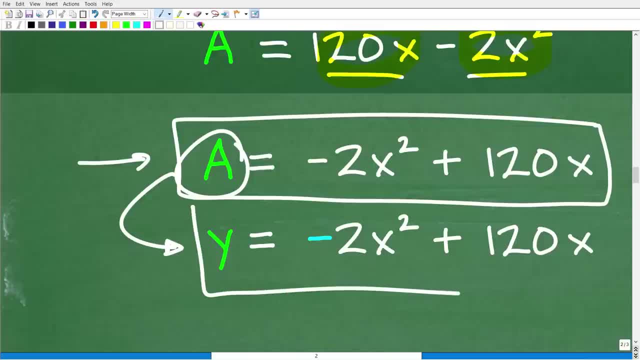 to minus 2x, squared plus 120x, because what we have right here is a quadratic equation. okay, we can graph this quadratic equation, and the graph of a quadratic equation, hopefully, you know, is a parabola. okay, it's some sort of parabola. now, what type of parabola is this? Well, there's. 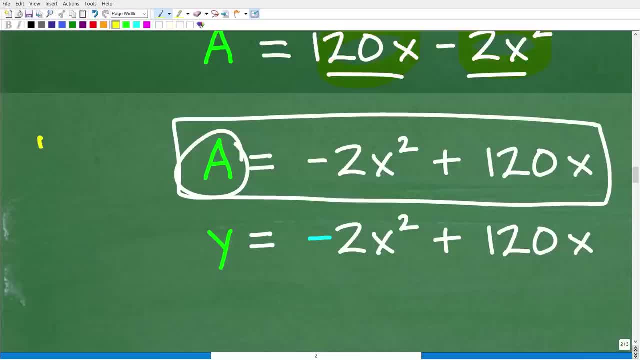 two types of parabolas. a parabola is a u-shaped kind of a graph. again it's the graph of a quadratic function. so we have happy parabolas and then we have parabolas that are sad to be. 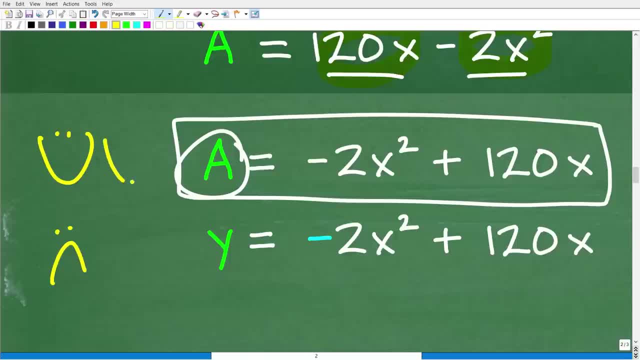 parabolas like this. so how do we know if we have an up parabola like this or a down parabola like that? Well, the way to know is to look at the sign of the leading coefficient. okay, so, in other words, we go to our x squared and if it's negative, well then we have a sad 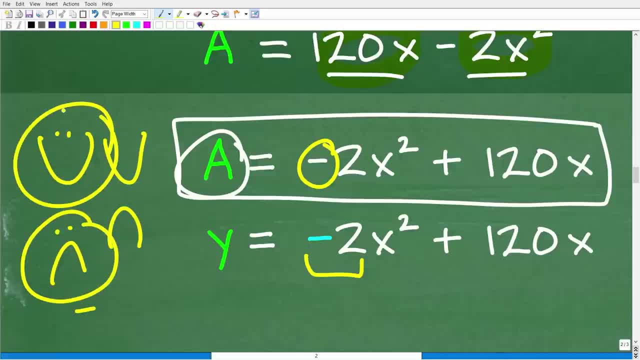 parabola. if this was a positive number, we would have a happy parabola, okay, so hopefully you remember that and I'm going over a lot of algebra here. if you're struggling with quadratic equations, parabolas, all this type of stuff, I will give you some specific recommendations here. 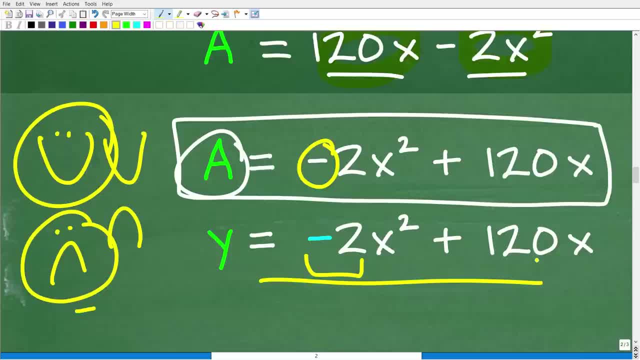 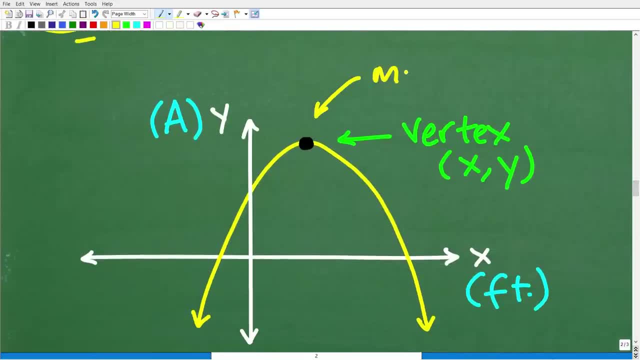 in just one second. but what we have again, if we were to graph this is some sort of sad parabola. and this makes sense because we are looking for the maximum. okay, you can't have the maximum like this if you have a happy parabola. 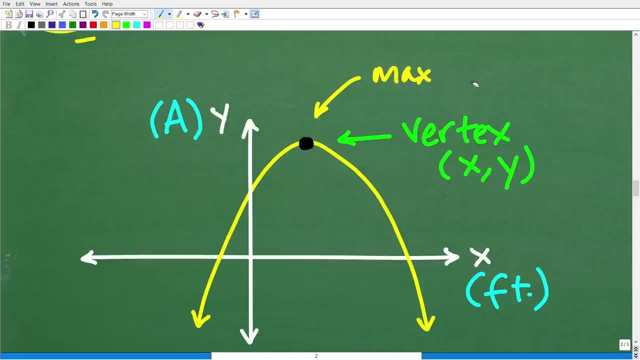 you would be looking for the minimum. okay, a upside down parabola like this. this is where it maxes out. all right, so again, what is x? Well, x represents the feet. okay, the amount of feet for the width of this fence. that's what the x variable represents. so that's the feet, and then 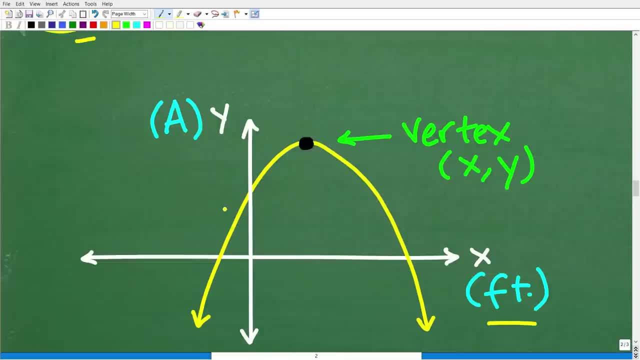 y represents the area, okay, of this respective enclosure. all right, so what we want to do is figure out how many feet- okay for our width should we have. there is a particular value, okay that we want to figure out, and that amount is going to correspond to the maximum area. so, really, what we're talking. 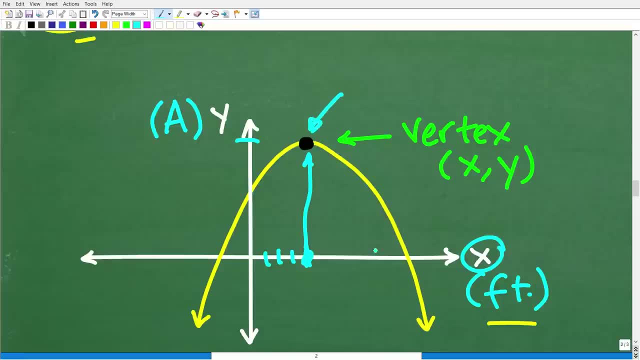 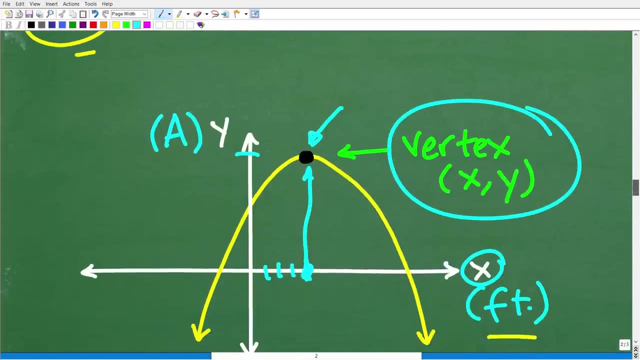 about is finding the maximum or the very top of this parabola, and that is a specific xy point called the vertex. Okay, so this is what this question now is all about: how do we find the vertex of this function right here? well, we're going to go ahead and get into a decent amount of algebra and again, 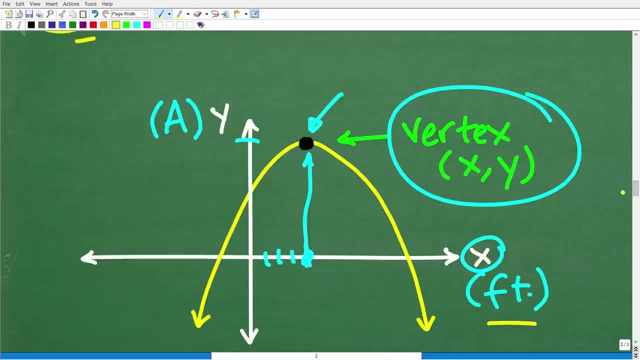 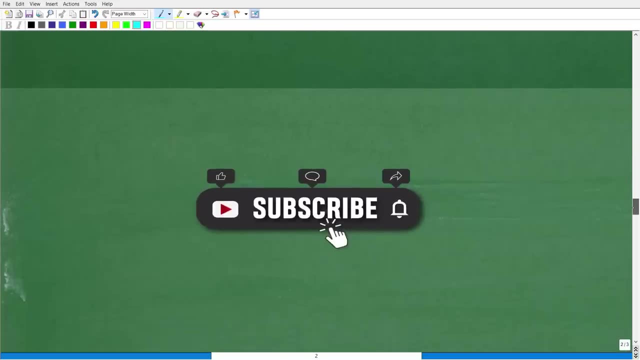 if you need help with this, don't despair. I will give you some very good recommendations, but let's go ahead and get into this right now. Okay, now, before we look at exactly how to find the vertex of a parabola, let's have a quick look at this, which, of course, is an invitation for you. 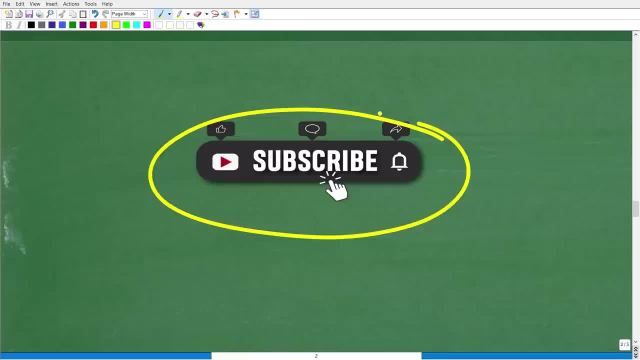 to support this channel And to support this channel and what I'm trying to do, which, of course, is reach as many people as possible and help them in mathematics. well, I can't do that unless I get help from people like yourself. Now, the way you can help me out is simply hitting that subscribe button. it really 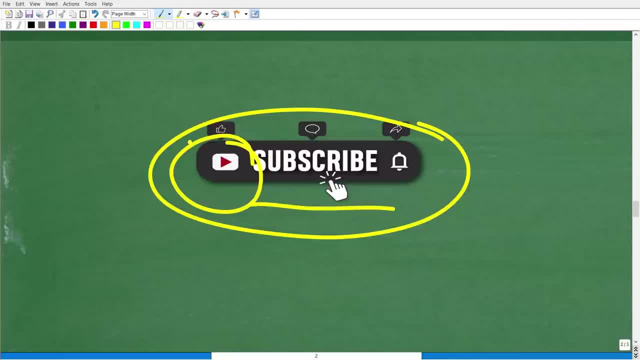 does a lot with that YouTube algorithm, and if you're going to do that, hit that notification bell as well, so you can get my latest videos. Now, the stuff that we're doing in this particular video- parabolas, quadratic functions and so on- is going to help you out, and I'm going to 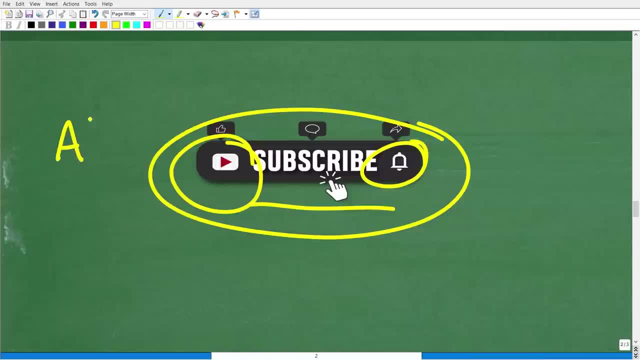 leave links to all my main full courses, which, of course, include Algebra 1,, Algebra 2, and other courses. you'll find those in the description, but I also have a ton of additional videos on my YouTube channel that can help you out with this stuff as well. Alright, so let's go ahead and 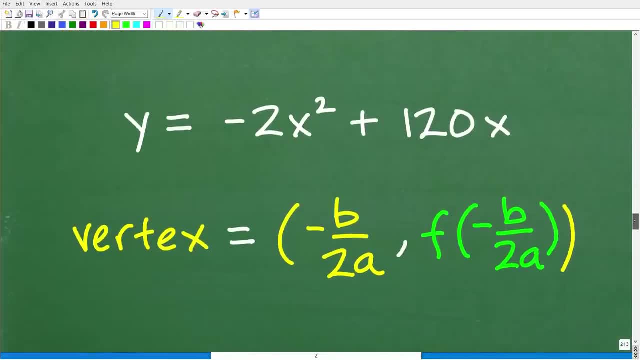 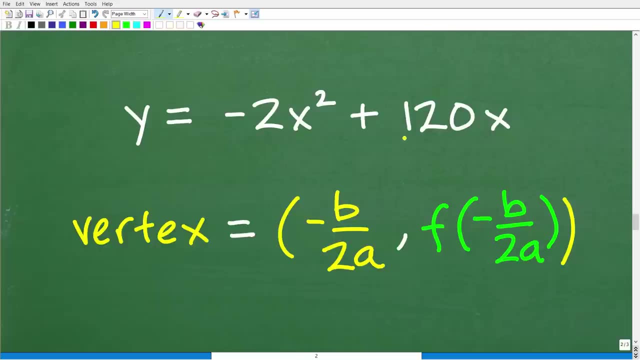 finish this problem up, and the next thing that we need to do again is to figure out the vertex of this quadratic function. So we have: y is equal to minus 2x, squared plus 120x. well, to find the vertex right, which, of course, is the top of this. 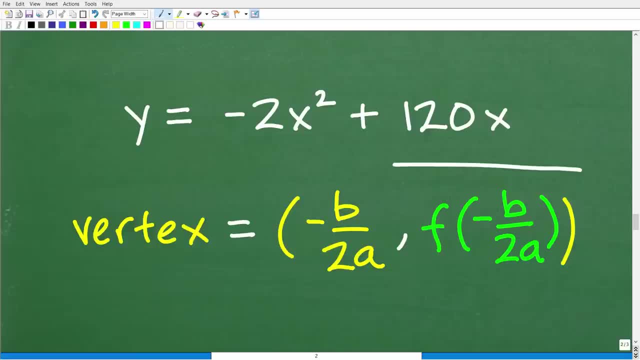 parabola. all we need to do is use this formula right here. Okay, so the vertex is equal to minus b over 2a. this is our x coordinate for our vertex, and our y coordinate is f of minus b over 2a. 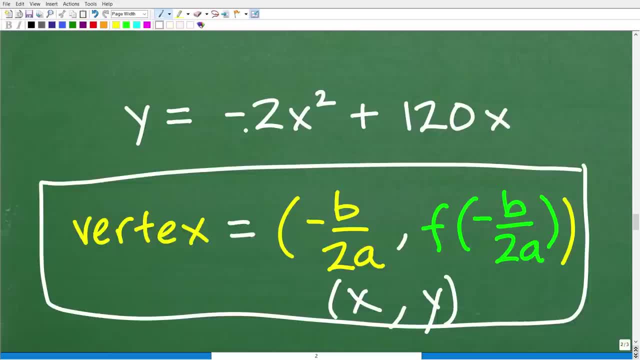 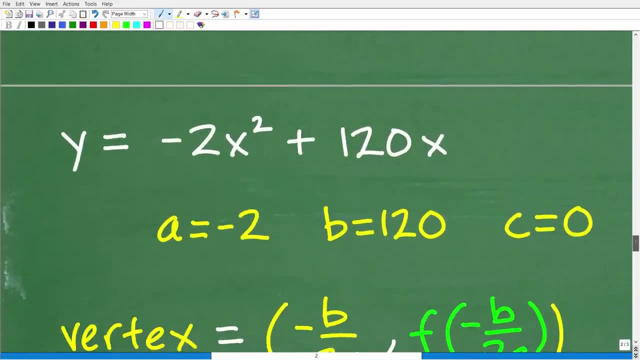 this x coordinate and then that answer we're going to plug in to the function and then we'll get the y coordinate. So let's go ahead and see how this is done. this is not that difficult, Alright, so we have our a, b and c values Now, the a, b and c values that we're talking about. 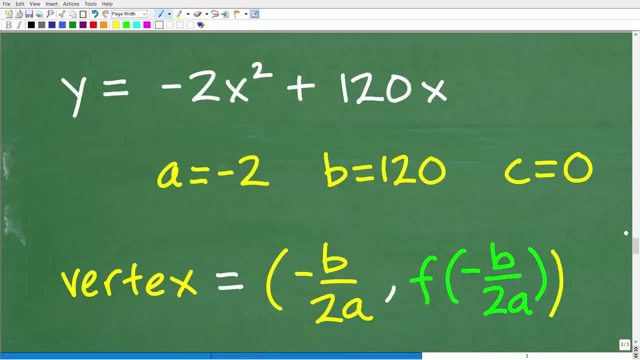 are the same a, b and c values that we use with the quadratic formula, if you're familiar with the quadratic formula. So the leading coefficient in this case it's negative 2, this is our a value. the x term is our b value. of course. that's 120, so a is negative 2.. Now we don't need c here for. 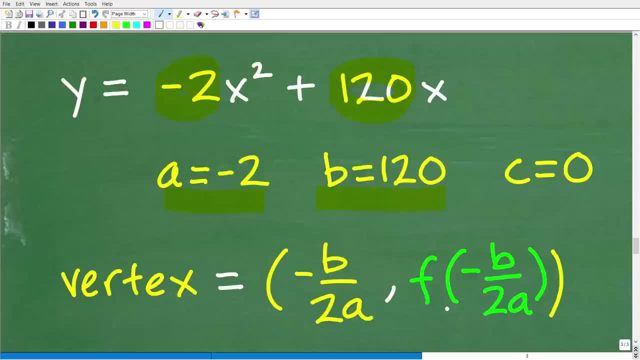 the vertex. but if we wanted to use the quadratic formula, you might be saying: hey, there's no c here. well, we could just say plus 0, so c could be equal to 0, but all we need to figure out the 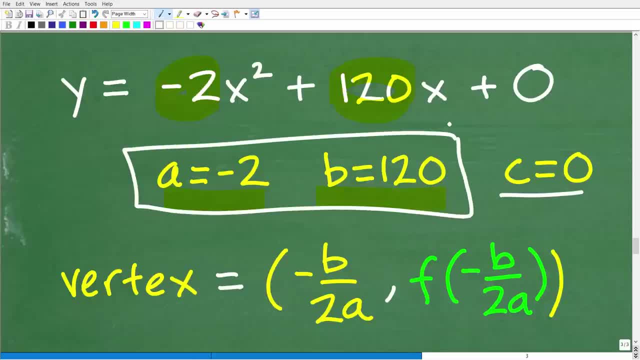 vertex is our a and b values. Alright, so this is pretty much just a substitution kind of scenario. we have b and a, so we're going to plug in a negative 2,, right here, and for b we'll plug in a 120, and let's go ahead and get our x component. 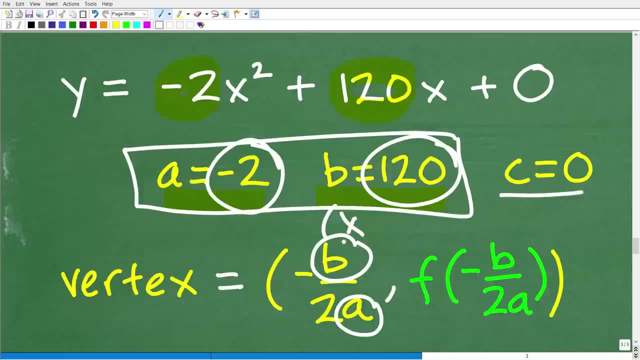 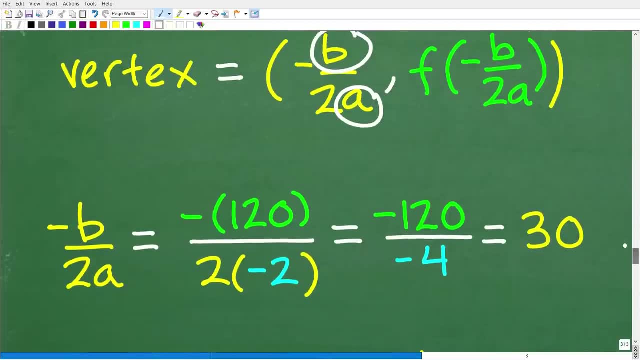 or x coordinate for the vertex first, and then we'll go back and get the y coordinate Again. don't let this formula scare you. this is not that difficult, Alright. so minus b over 2a is going to be negative 120 over 2 times a, which, of course, a again is negative, 2, and b is 120,. 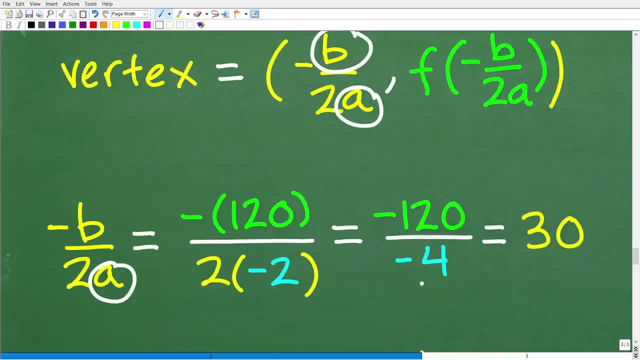 so we have a negative 120 over 2 times negative 2, is negative 4, so negative 120 divided by negative 4,, of course, is a positive 30. Okay, so we are almost done. that means for our vertex: okay, our x coordinate is 30.. Now 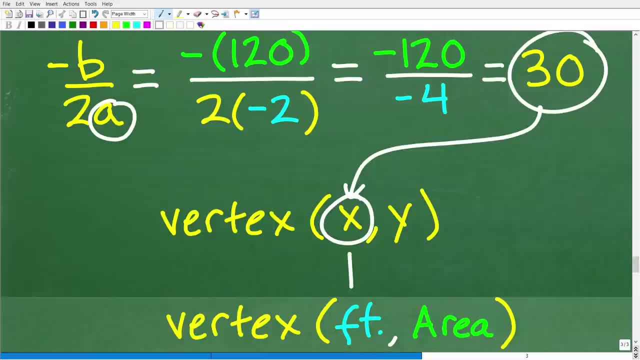 remember our x axis. our x variable represents the feet. okay, in terms of the dimension here for our width on our lovely rectangular plot. okay, so we almost are done. but remember the y component of our vertex represents the maximum area, because that is the question. So we still. 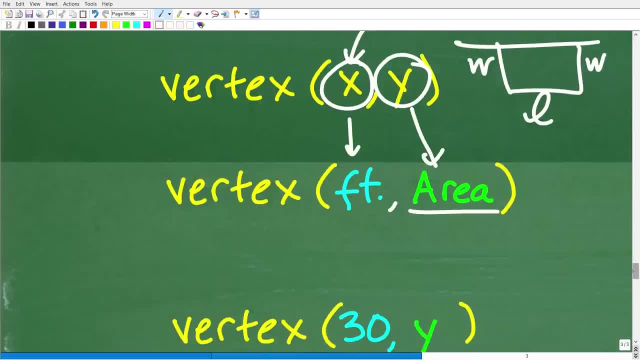 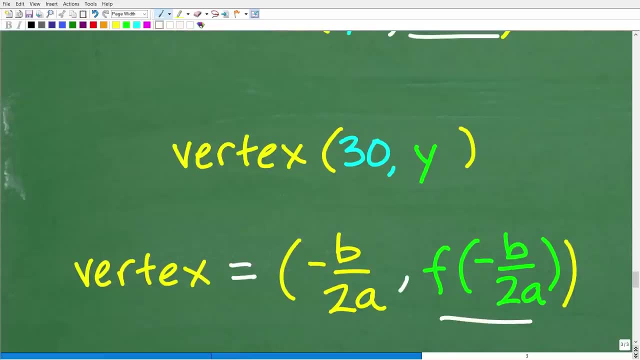 have to figure out the y, which, of course, is the answer to this problem, and to do that, what we need to do is do this part of the formula, which is f, of minus b over 2a. All that means is that: 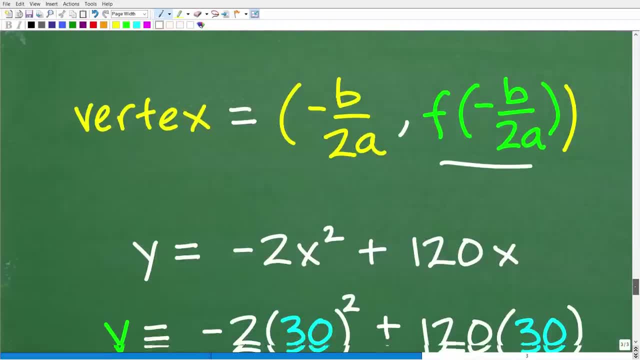 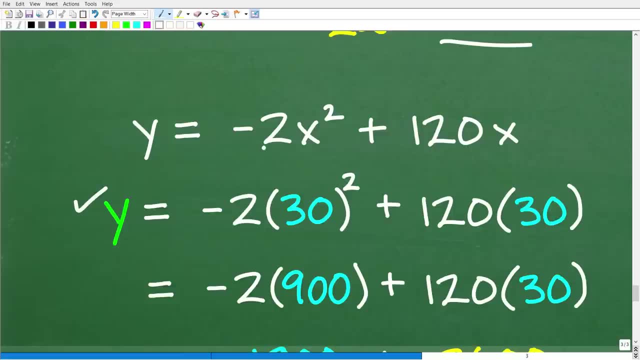 we're going to take our x coordinate and plug it into the function, okay. so when we do that, we will get our y. so minus b or minus 2, negative 2x squared, excuse me, plus 120x. so we are going to plug in a 30 right here, okay. 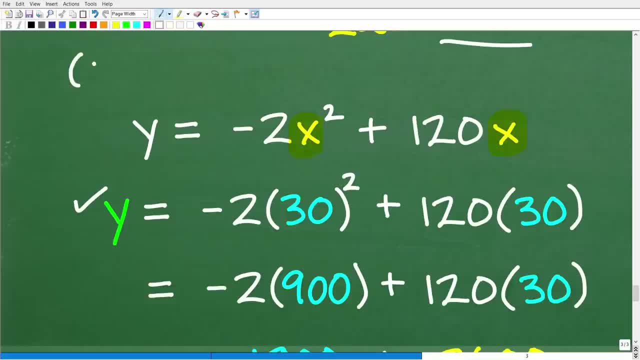 because this 30 is the x coordinate for our vertex, right? so you got to get this first, and then we're going to plug in our value- which of course is 30, into our equation to get y. All right, so we have 30 squared, which of course is 900 times negative 2,. 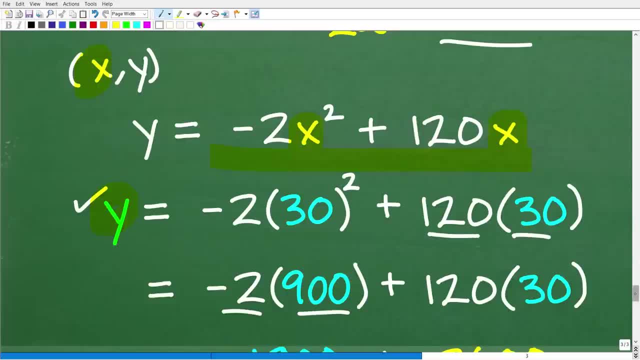 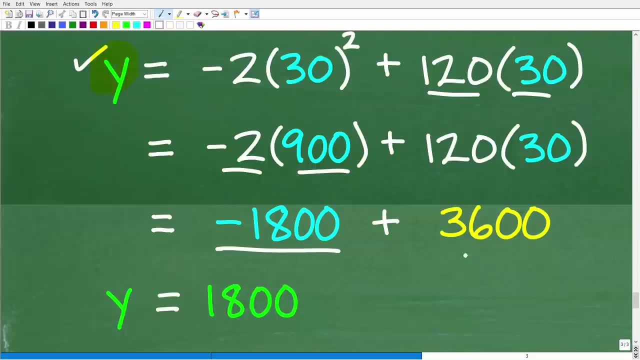 and then 120 times 30, and we'll do all this number crunching. this is not that difficult. so negative 2 times 900 is negative 1,800, plus 120 times 30 is 3,600, and when we add these, 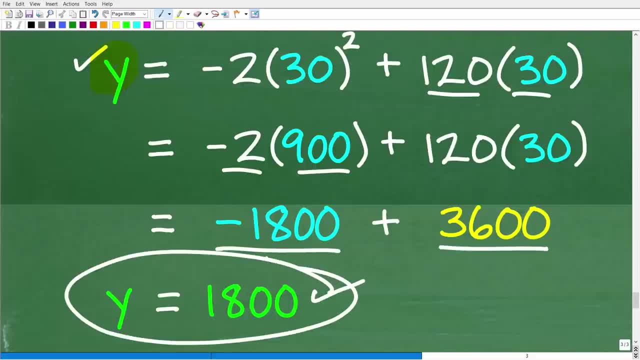 together we get 1,800.. All right, so that is our actual maximum area. okay, 1,800 square feet, All right. now again, you could go back and get the actual dimensions of this rectangular plot. but that is not the question Now. I'm going to show you another way that we can use calculus. 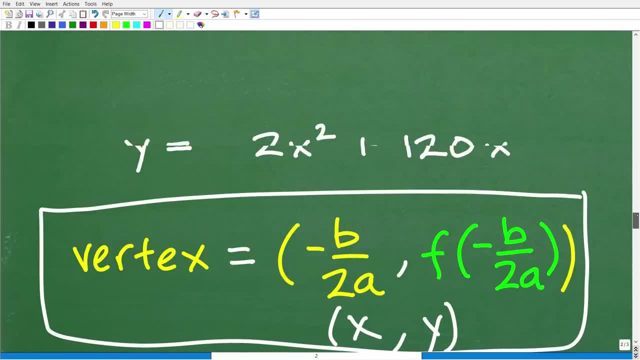 to solve this problem. So let's go ahead and do that. So let's go ahead and do that. So let's go back up here and revisit our parabola. okay, This is going to be a quick micro lesson. 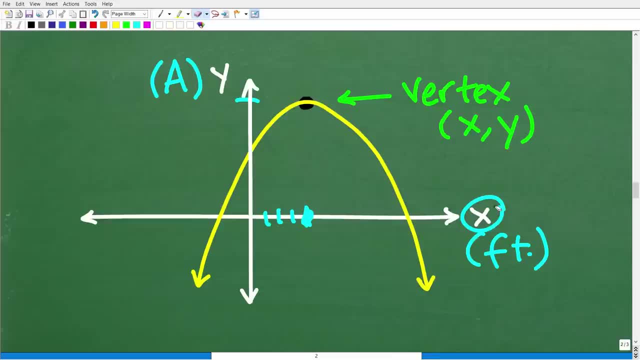 on calculus. and how can we find the vertex, the very top of this point, using calculus? Well, there's something called the derivative. all right Now. the derivative is a formula that tells us the slope of anywhere along a curve. all right, So slopes, if you know how to graph a line. 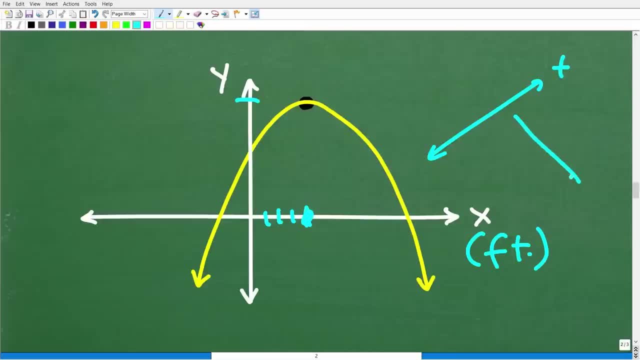 lines that are going in this direction have a positive slope, lines that are going this way have a negative slope, and then lines that are completely horizontal have a slope that is zero. okay, So if we look at this parabola here now anywhere, as we're kind of you know- 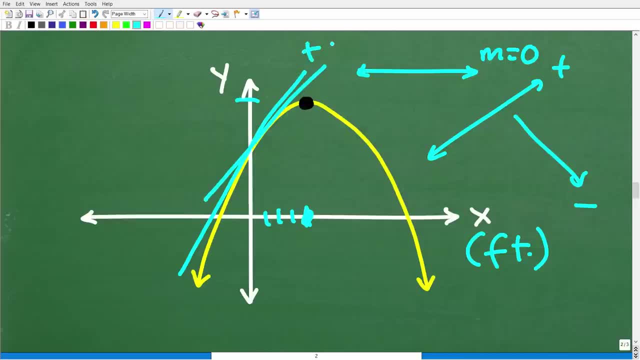 approaching this left-hand side of the parabola. the slope on the parabola is positive. Over here it's downhill, so it's negative, right, but there is one point where the slope is zero, okay, and that point is right here at the maximum. okay, That's where the slope is zero. 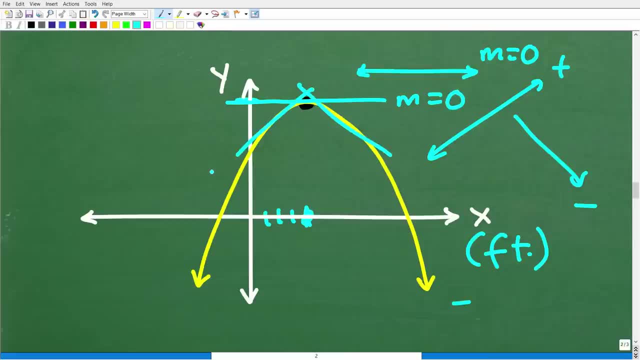 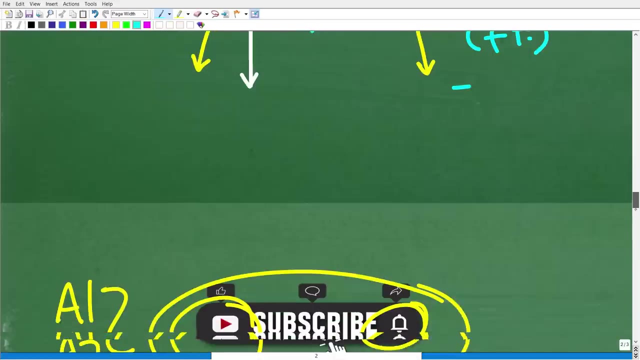 and then it kind of goes down here, downhill there and then uphill right there. So if we can figure out along this parabola where the slope is zero, well that indeed is our x value for the vertex, and this is so easy to figure out when you know a bit of calculus. All right, So I'm just going. 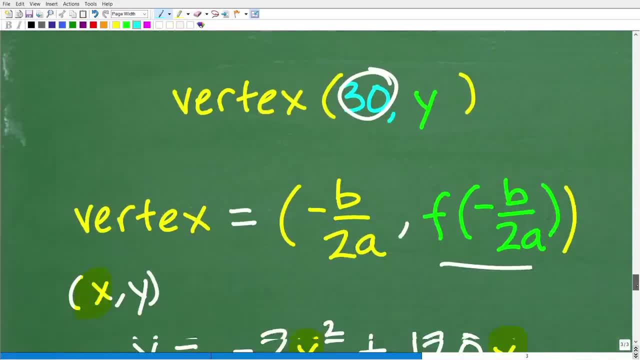 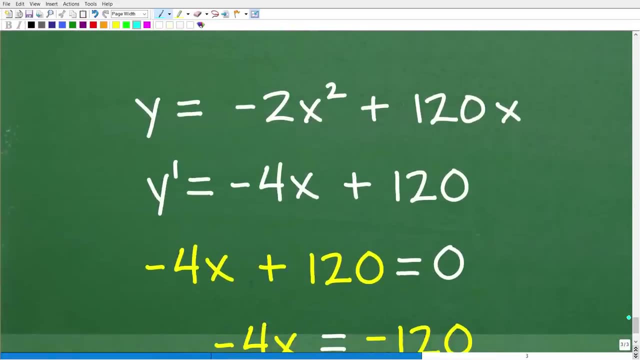 to show you this real quick. I'm not going to fully explain this because this video has already been a little bit long, but this is definitely worthy to see. All right, So here is our function. our quadratic function, y is equal to minus 2x, squared plus 120x. Okay So, 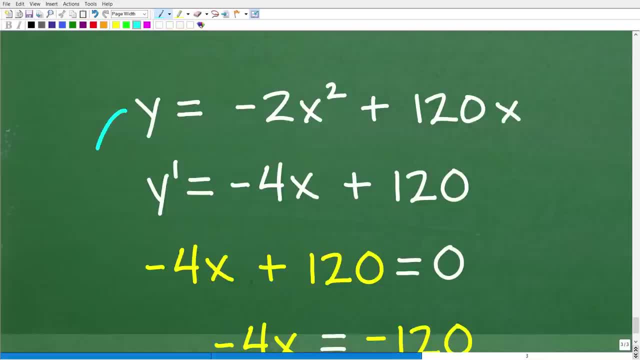 what we're going to do here is get something called the first derivative, or y prime, in calculus. Now, this is not that difficult. okay, The first derivative is the formula for the slope. okay, This is the slope along our parabola. 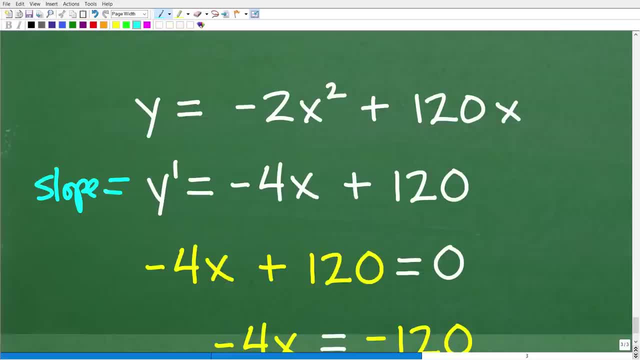 Okay, Now of course I'm going very quickly here in terms of explaining calculus, but the way we find the first derivative is: I'm going to take this 2. I'm going to multiply by that negative 2.. So 2 times negative 2 is negative 4.. Then I'm going to drop this power down: 1. So 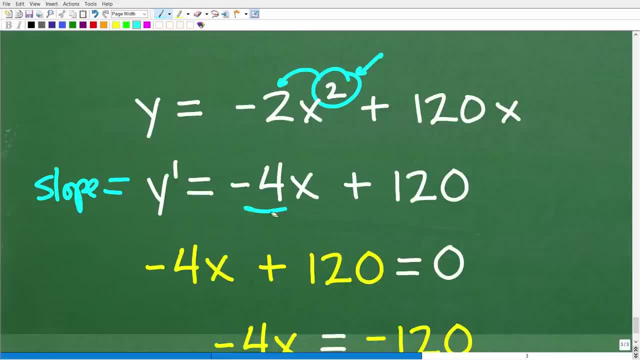 instead of x squared, I have x to the first. All right, This is how we find the derivative. You can see, it's not that difficult when I'm doing, and then over here I'm going to do the same thing- I have x to the first, I'm going to multiply by that number, So that's 120, and then I'm going. 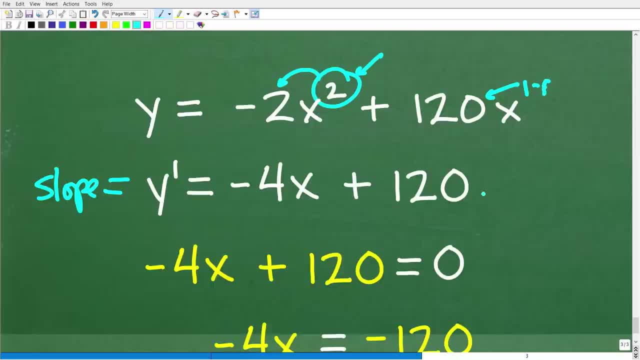 to decrease the power by 1.. So that's x to the 0 or just 1.. Okay, So you just decrease the power by 1.. This is a basic rule in terms of finding the first derivative of polynomials. Now, this is a. 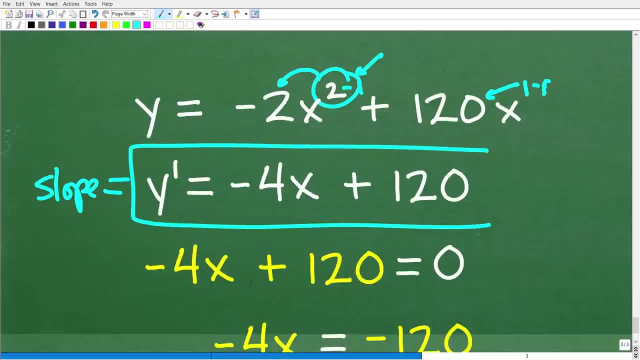 huge topic, as we are talking about calculus. but anyways, this is the first derivative. Okay, Now, what do we do with this? Well, this is the slope, and we want to say: hey slope, when are you equal to maximum? So what we're going to do here is set this first derivative, negative 4x plus 120, equal. 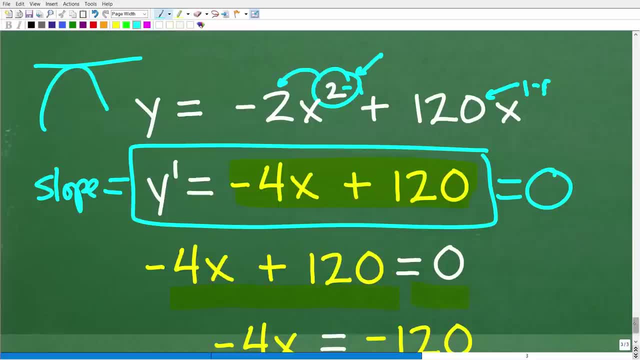 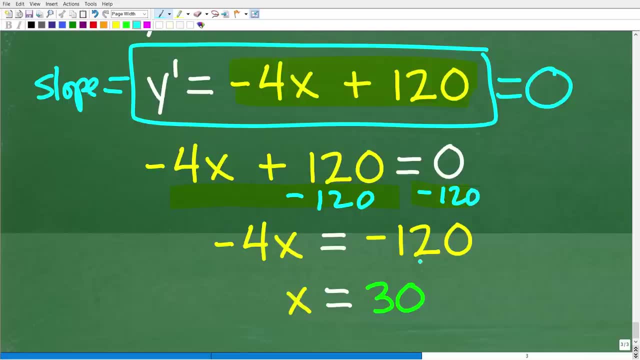 to 0, and we're going to solve for x. Now let's just go ahead and do this real quick. So we're going to subtract 120 from both sides of the equation. I have negative. 4x is equal to negative.